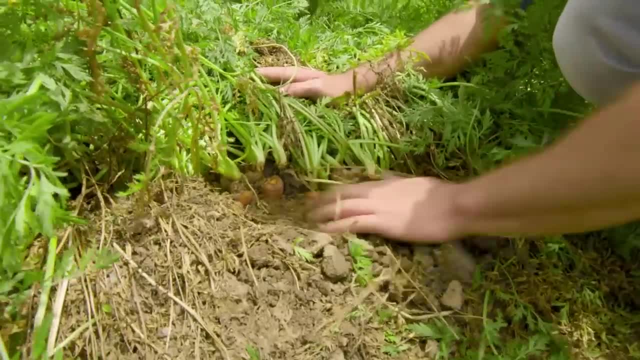 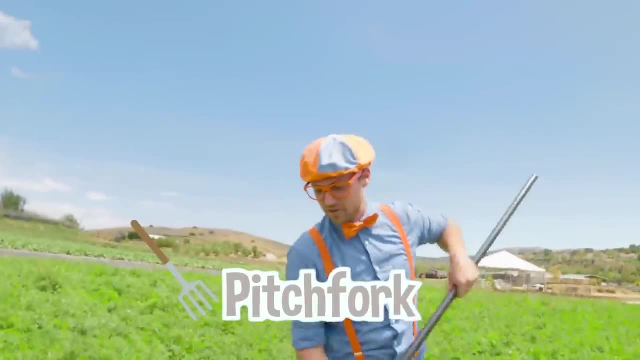 Yeah, See all this orange. Yeah, Those are carrots, But they're pretty stuck under there. So let's take this giant pitchfork- Whoa, Looks like a small fork, but way bigger- And then let's loosen up the soil. 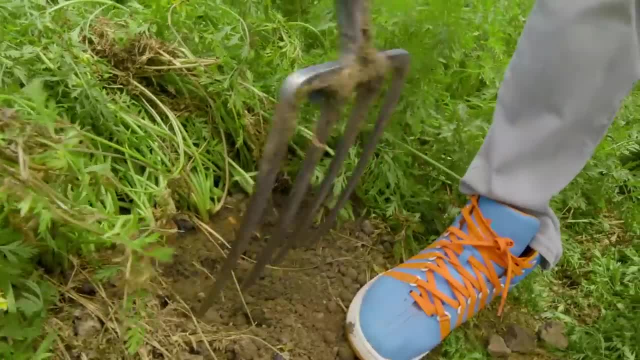 Oh, That's how you get a big, big carrot. You turn it around like this And then it's ready to go. Look at this, It's a very big carrot. Let me take a look. Okay, Whoa, Awesome. 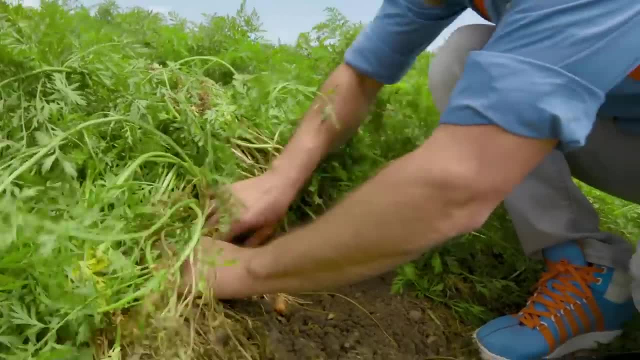 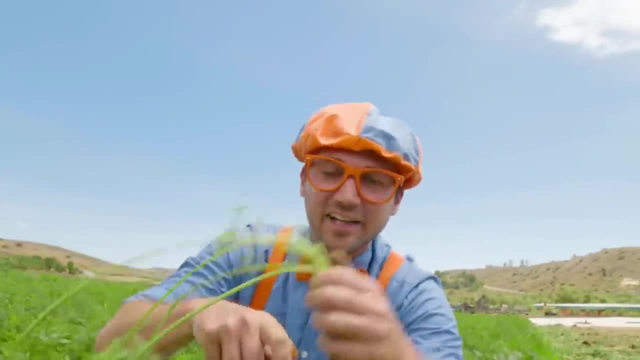 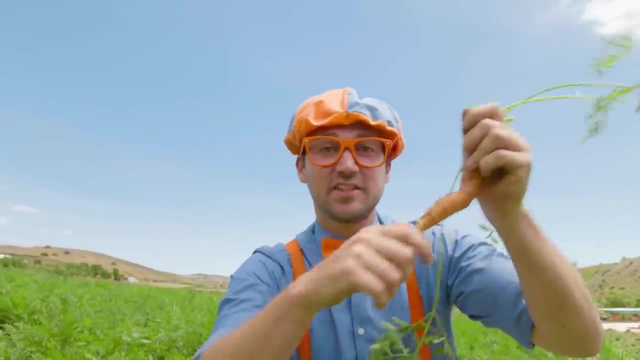 Wow. And then we need to pick a carrot. Hey, There's one right here, Whoa, Check it out. We got a carrot, Whoa. Yeah, That's cool. I love carrots. They're the color orange. I love putting them in my salads, my carrot cake. 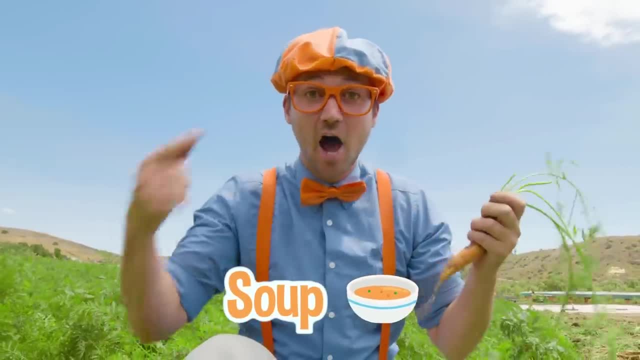 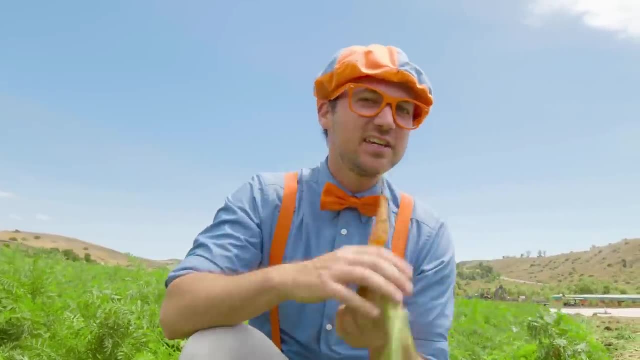 even some soup. They're so yummy And they help your eyes be able to see at night. Whoa, pretty cool. Hey, and actually there's an animal that really loves to eat carrots. Can you think of what animal that is? 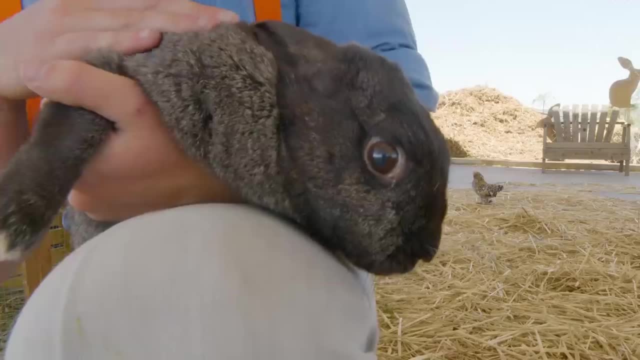 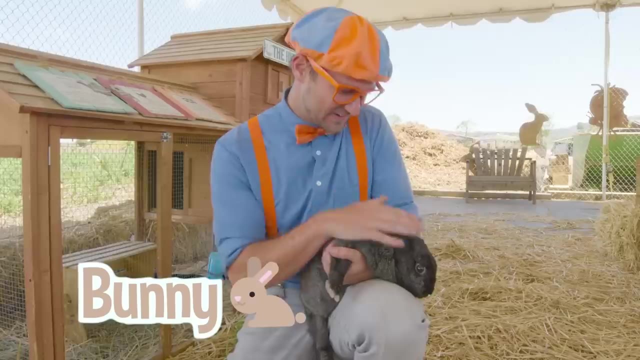 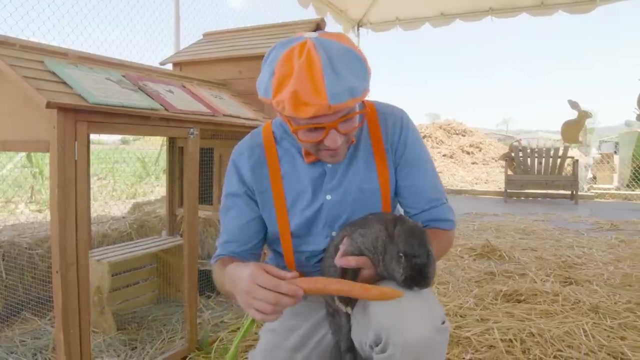 Huh, let's go find it. Oh, cute bunny. Look, look, it's a cute bunny. Wow, this bunny's name is Andy. Oh, I wonder if Andy wants a carrot from earlier. Here you go, Andy. 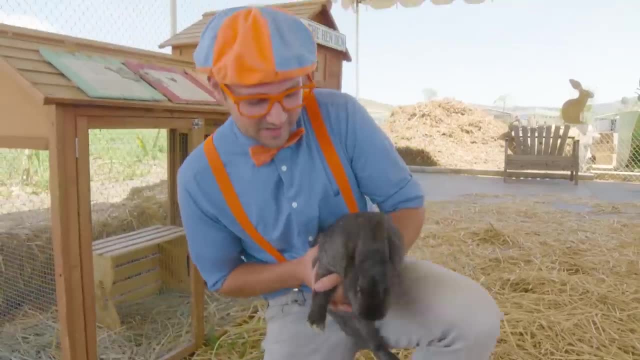 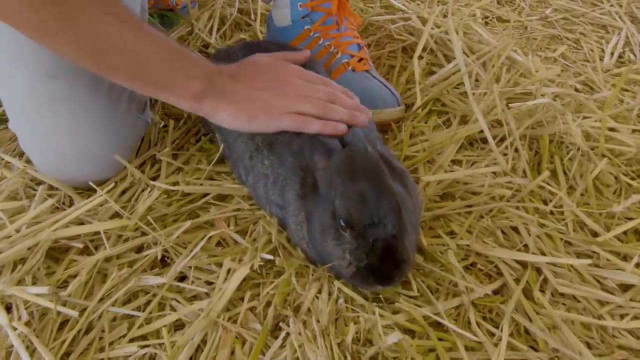 Maybe Andy's not hungry. That's okay, Let's put Andy down. There you go. All right, there you go, Andy. Whoa, I love bunnies. They're so soft. Hey, this is peanut butter, And the other one: 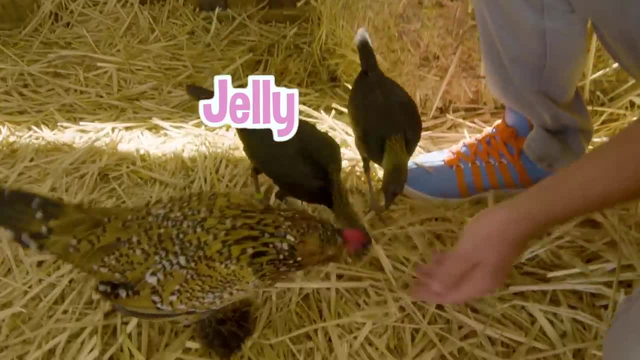 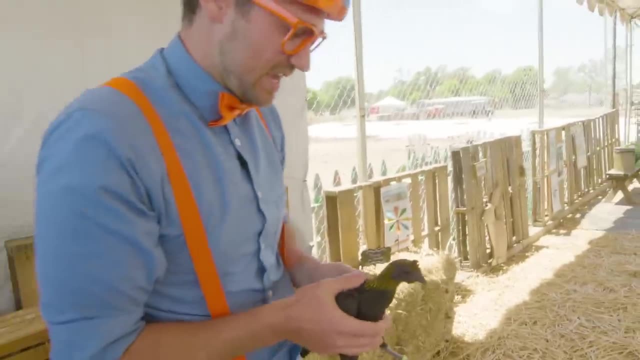 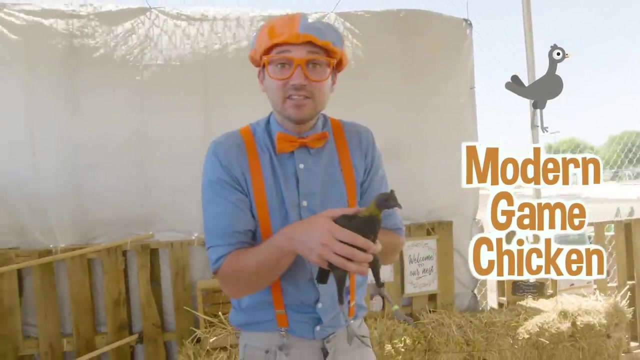 it's name is Jelly. Oh, here's another one. Oh, look at all those. Oh, hey, there you go, It's okay, yeah, Wow, do you see this chicken? This is a modern game chicken. Yeah, and they still lay eggs. 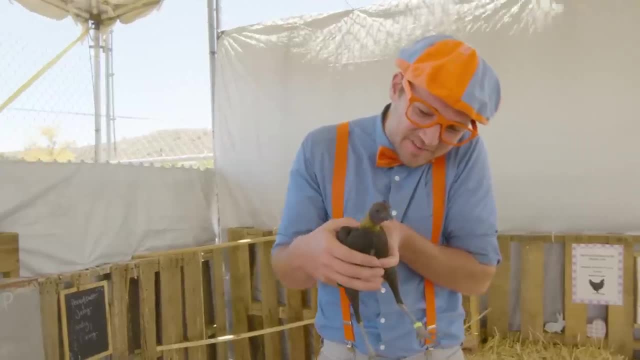 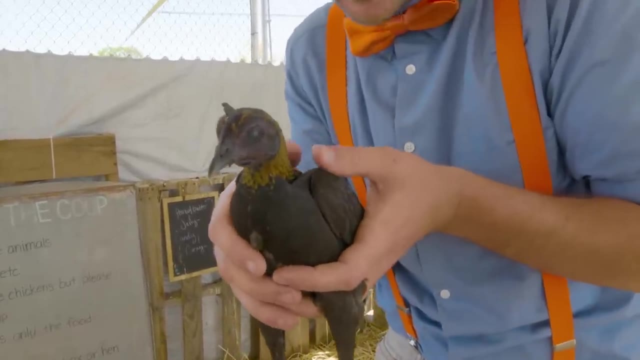 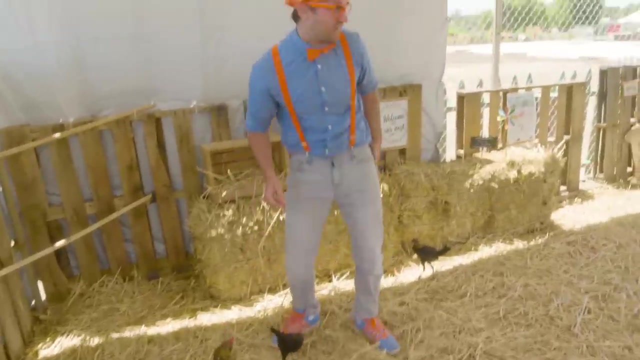 although they're really small. Yeah, look at them. Hey, they're so cute. Wow, Okay, let's put peanut butter down. So then peanut butter can eat some of the mealworms. Okay, there you go, Oh, and come over here. 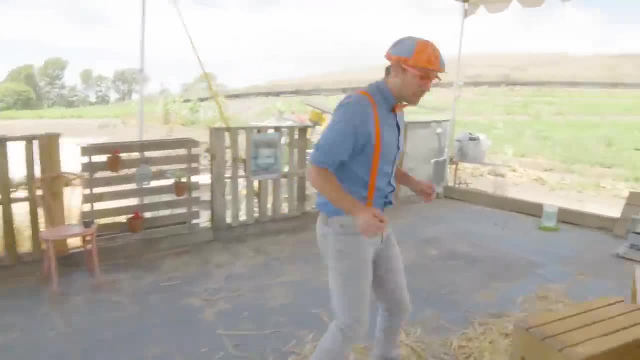 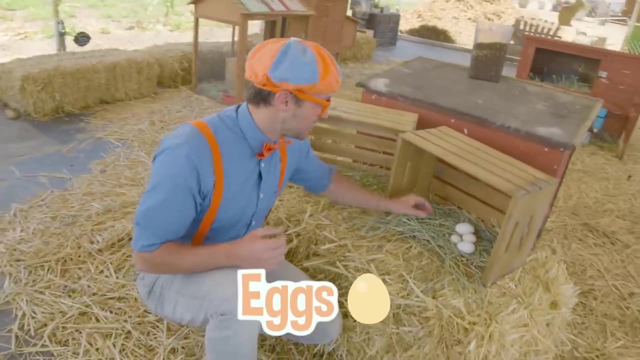 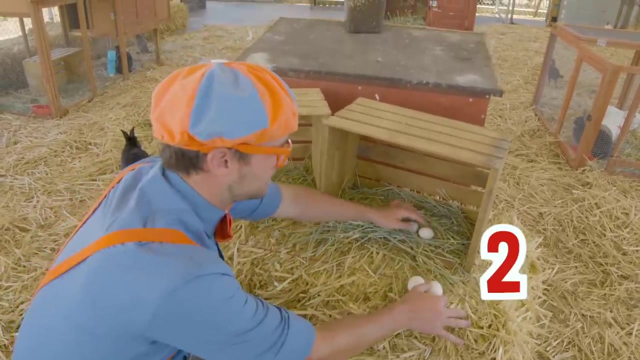 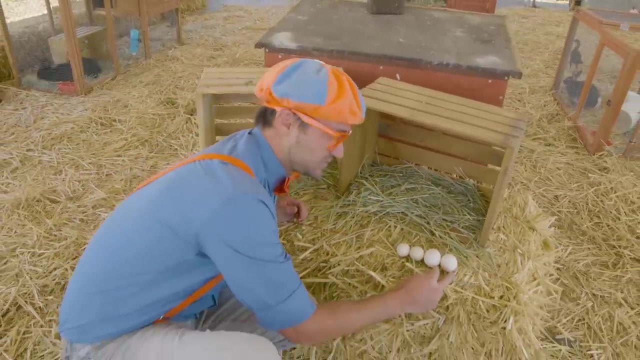 I have something to show you. Wow, right over here we have some eggs, Chickens, lay eggs. Wow, We have one egg, two eggs, three eggs and four eggs. These two are big eggs and these two are small eggs. 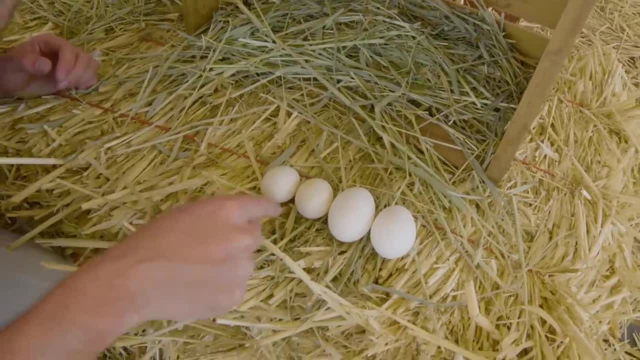 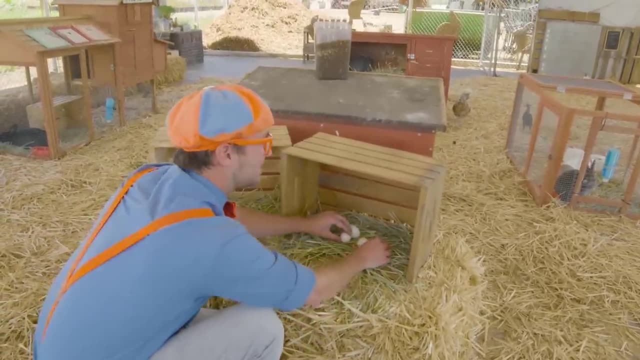 But these two weren't laid by the modern game chicken. These are still too big for those chickens. Okay, we'll put these eggs back right here and let's go check out the chicken some more. Oh look, Oh look. 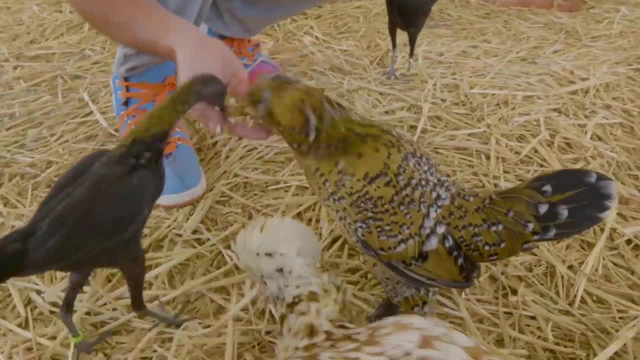 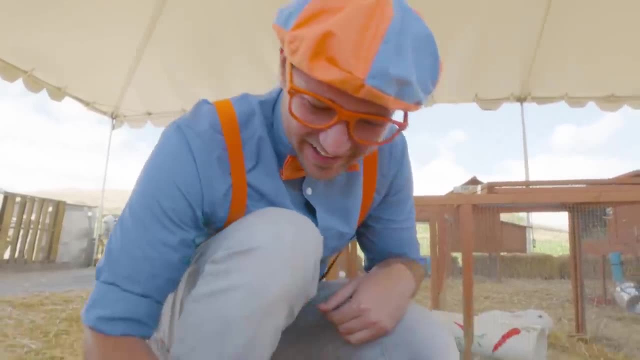 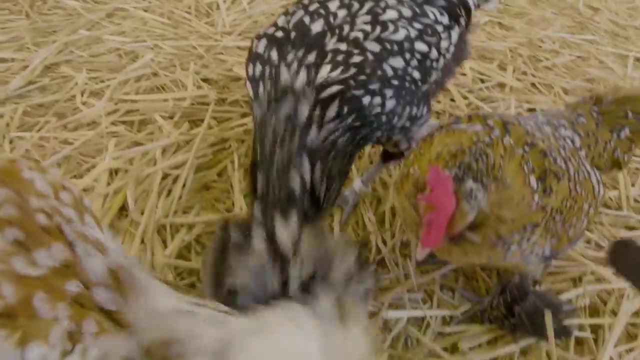 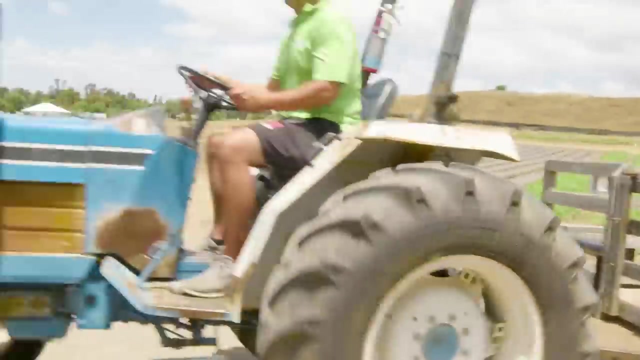 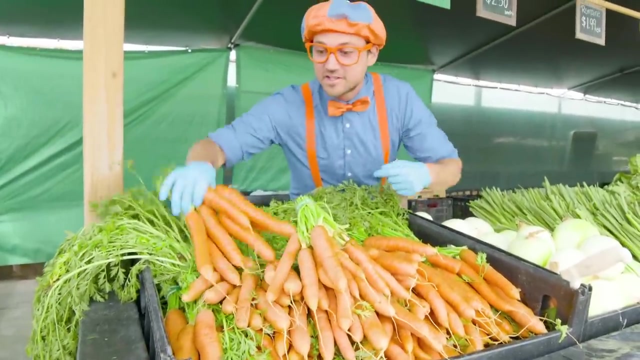 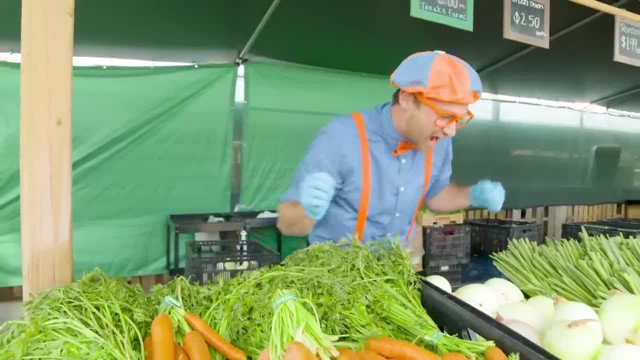 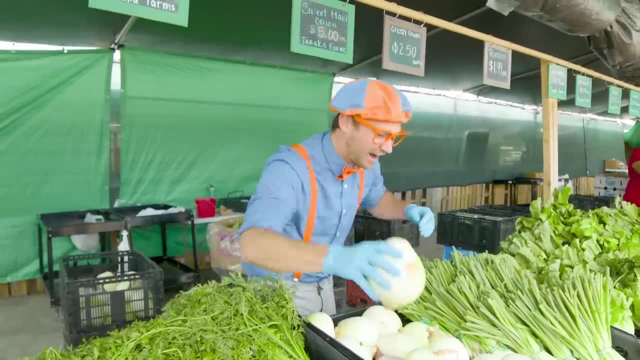 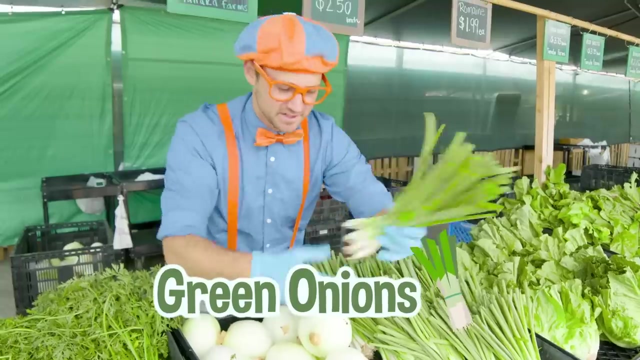 I love the color orange. It's one of my two favorite colors. Whoa, and these are onions. Wow, that is a big onion. And look at these. These are also onions, but these are called green onions. Yeah, they're both onions, but they look so different. 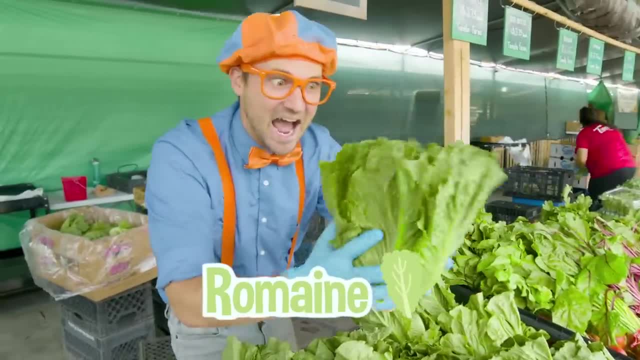 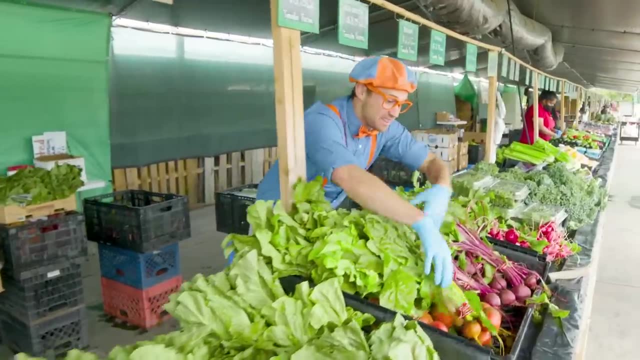 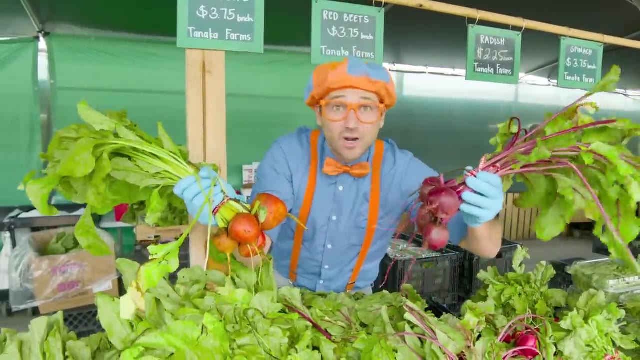 Wow, this is romaine. I love romaine. It's so healthy I like to put it in my salads. Wow, and these are beets. Whoa, these are golden beets and these are just beets. Oh look, check these out. 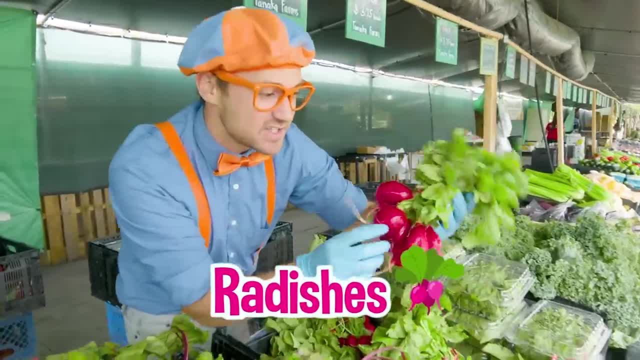 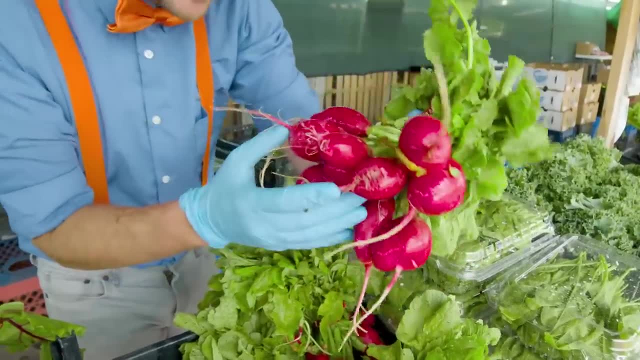 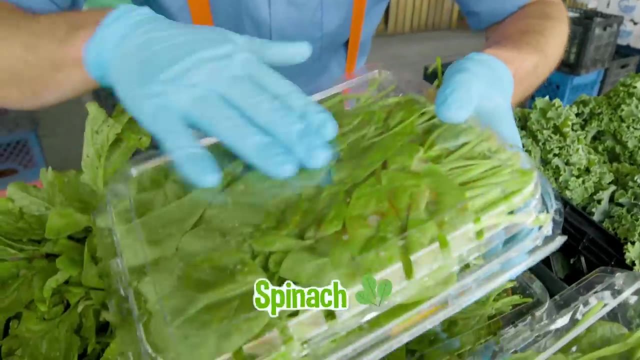 These are cute. These are radishes. Do you see the color? It's kind of like a pinkish red. Yeah, I like that color. Hey, and spinach. These are in a little case, a clear case. Yeah, spinach is green. 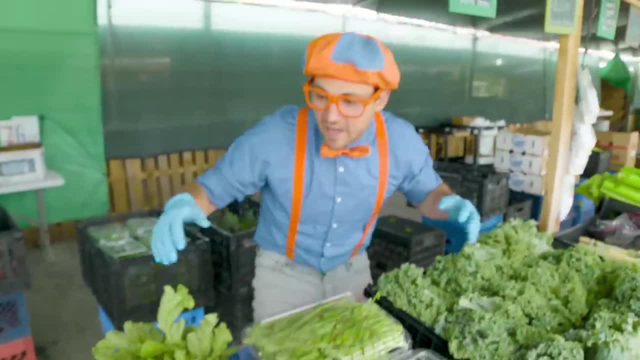 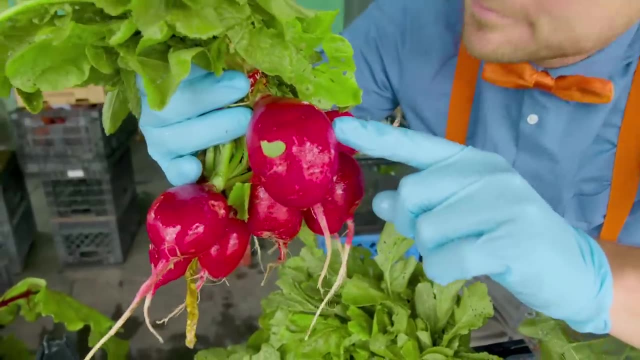 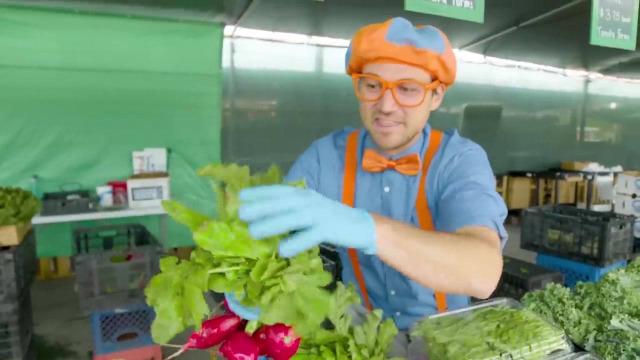 A lot of these vegetables are the color green, it seems like. Well, see the radishes. Yeah, the part that you eat is the pinkish red color, but up here this uses photosynthesis to grow the radishes and this is the color green. but you don't need the top. 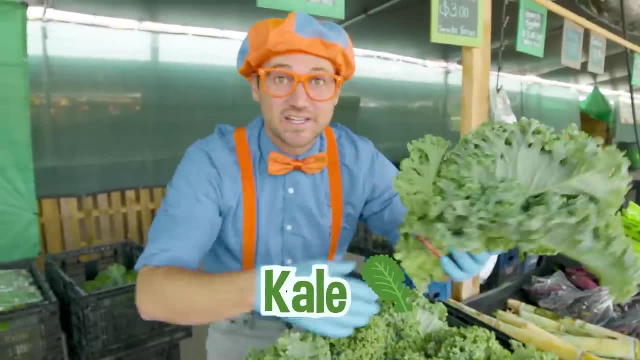 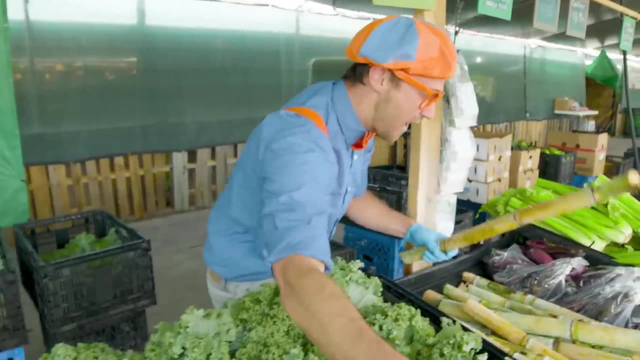 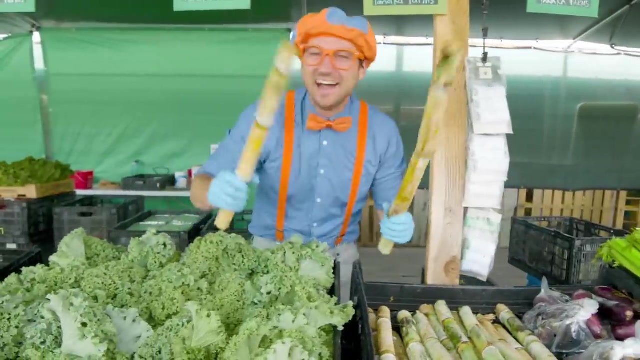 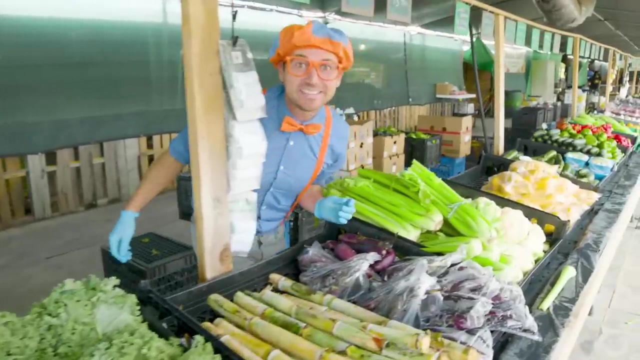 Wow, Wow, Kale. You should try some kale chips sometimes. Yeah, it's like normal chips, but healthier. Wow, Are these drumsticks? Nope, these are sugar cane. Wow, That is so sweet. Wow, Japanese eggplant. 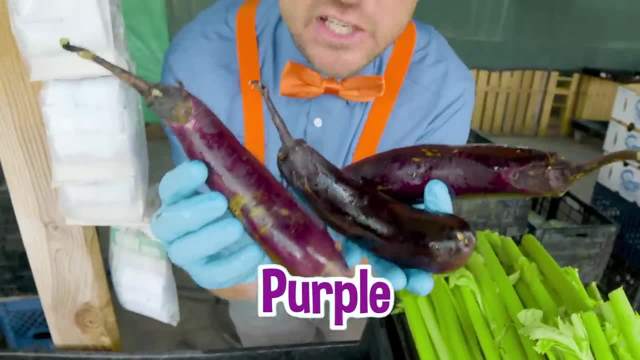 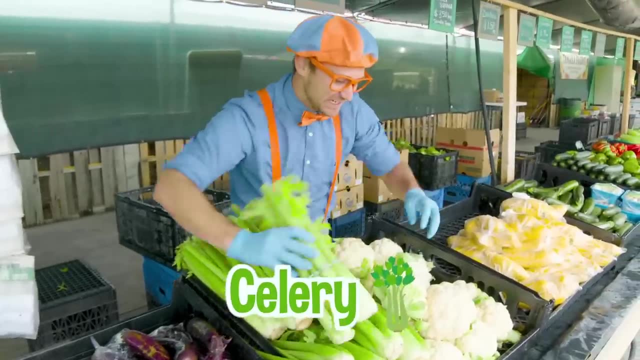 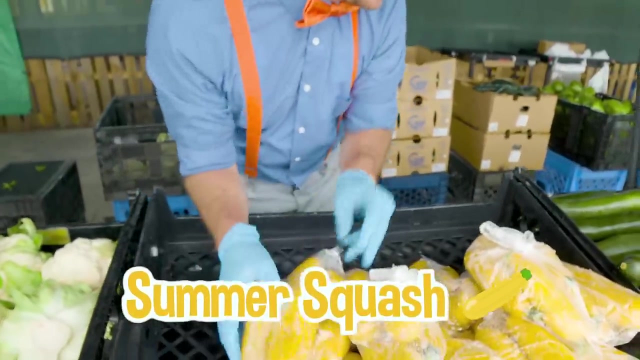 Wow, These are the color purple. It's a very dark purple. Wow, so cool and healthy. Oh, we got some green celery, We got some cauliflower Mm. Oh, can't forget about the summer squash, Yeah, Wow. and we also have some green bell peppers. 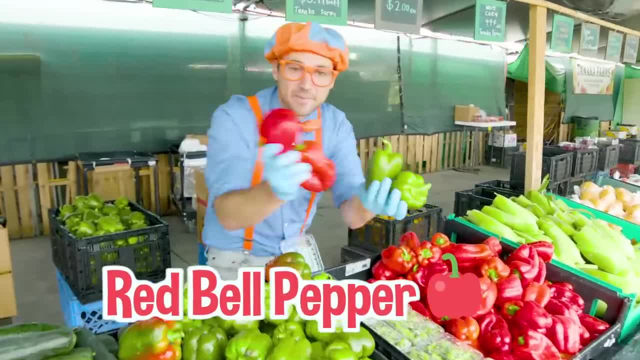 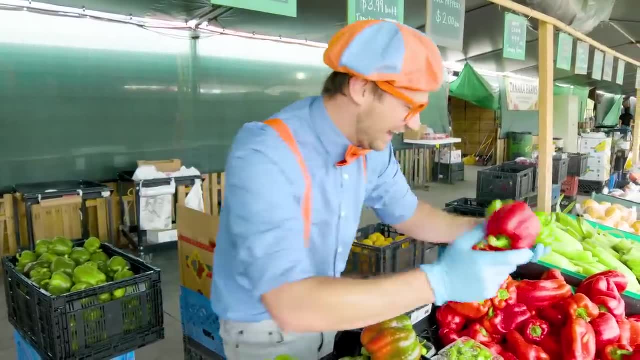 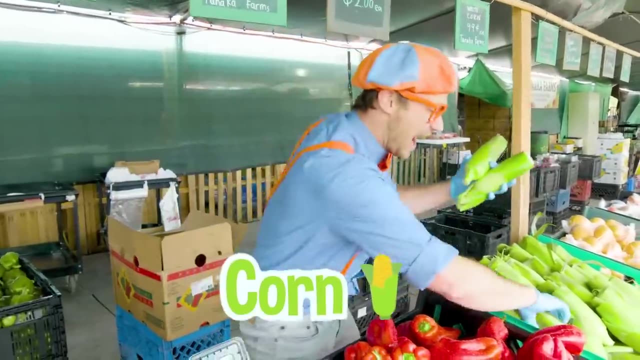 Yeah, right next to the red bell peppers, Check it out. Yeah, red green, Red green, Red green. We'll put those back just right there. And last but not least, we got some corn on the cob. 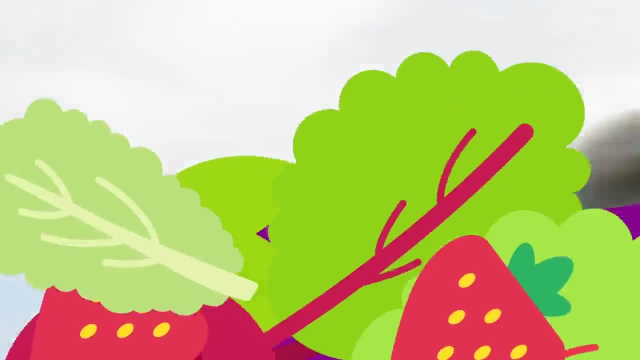 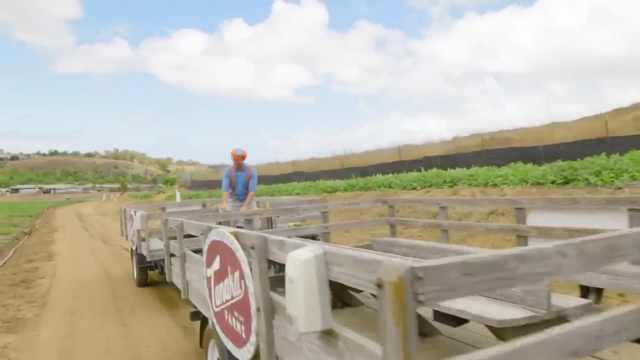 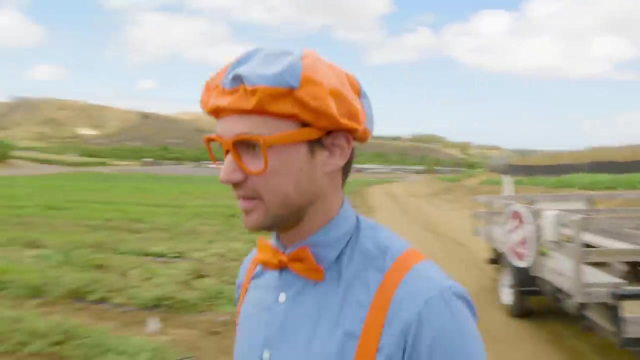 I love corn. All right, Blippi, we're here. Yes, I am so excited. Wow, I wonder what type of food this is. Okay, let's see. All right, We could go down this row right here. Okay, this one. 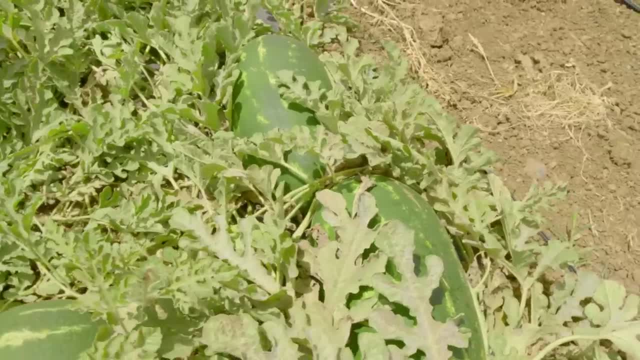 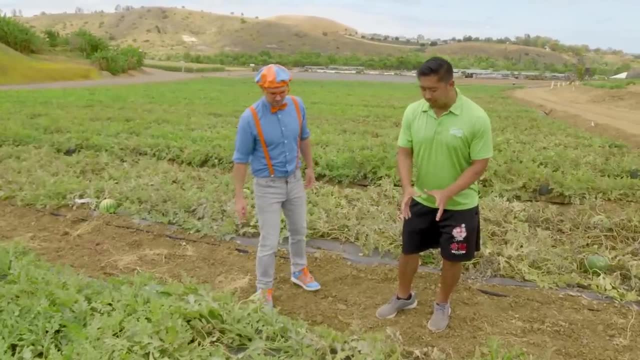 All right, Whoa, what are these? Those are watermelons. Watermelons, Wow. it looks like there's two different kinds. Yeah, there's these small round ones, Those are yellow watermelon, Okay, And then those big oblong ones. 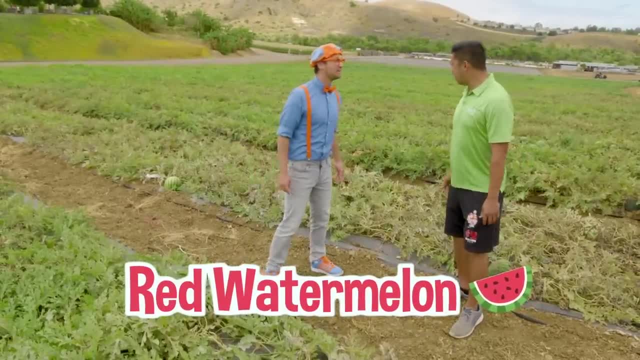 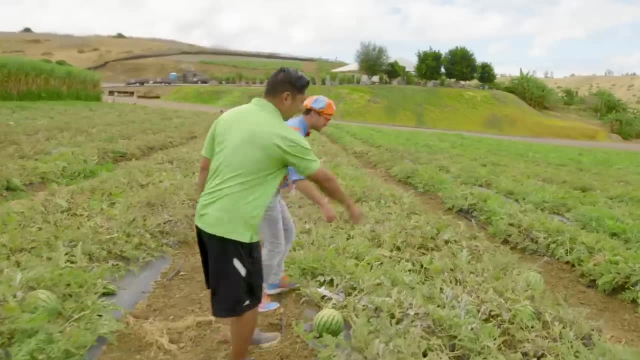 those are red seeded watermelon. Wow, can we pick a couple? Yeah, let's find some to pick. Okay, How about this yellow one right here? Okay, Right in the middle, This one, Yeah, Okay, how do you do it? 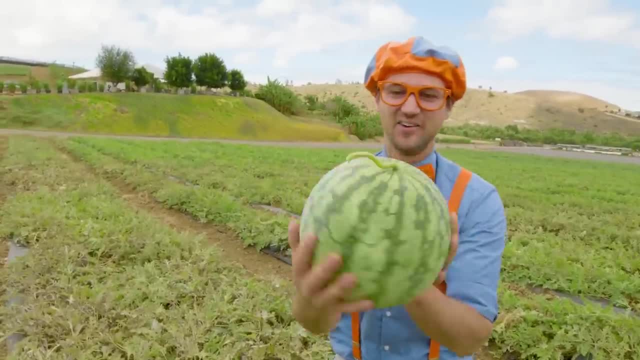 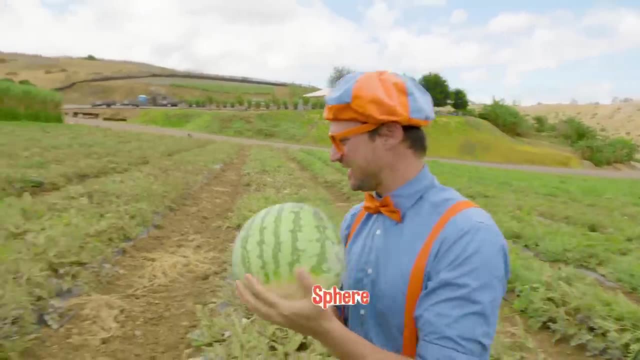 Just go in, it comes right off. When it's ready, it comes right off. Wow, look at it. This watermelon is a circle or a sphere. Okay, all right, Let me go. I'll go grab a red one. 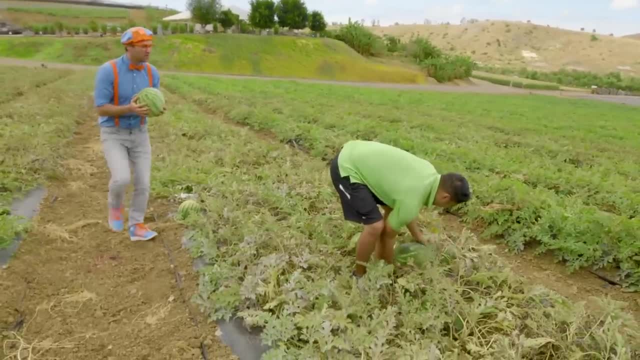 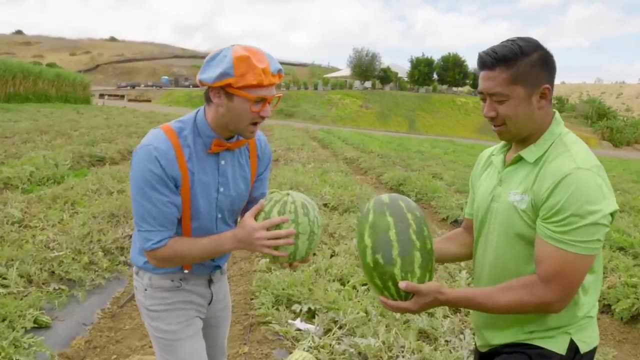 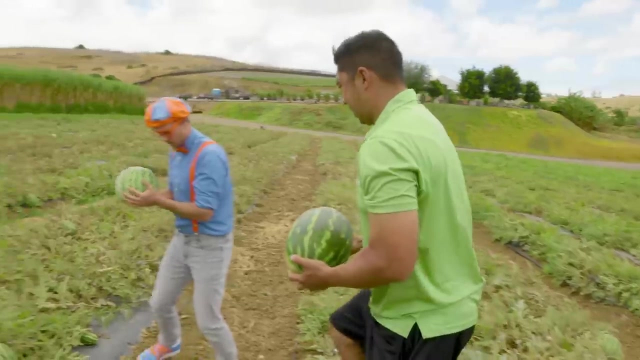 Okay, whoa, that's a big watermelon. Wow, what shape is this? Looks like a sphere to me, Yeah, kind of like a oblong sphere or an oval. All right, Now can we put them down right here? 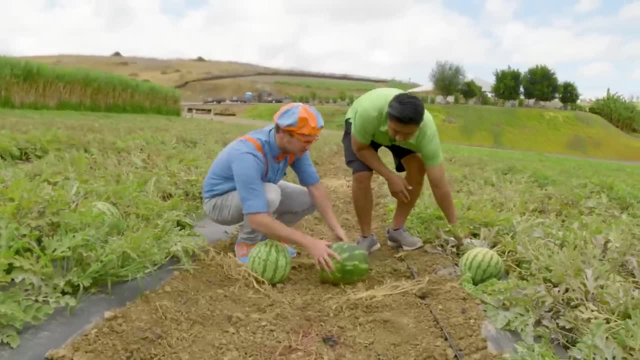 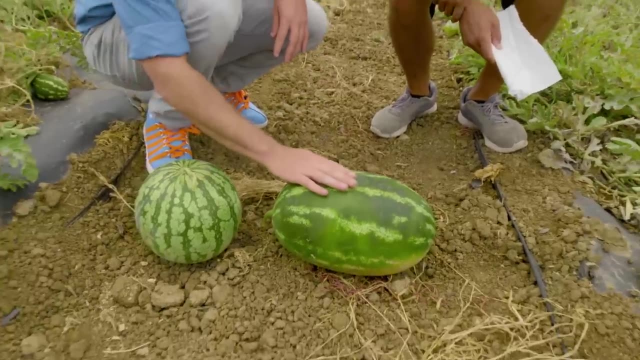 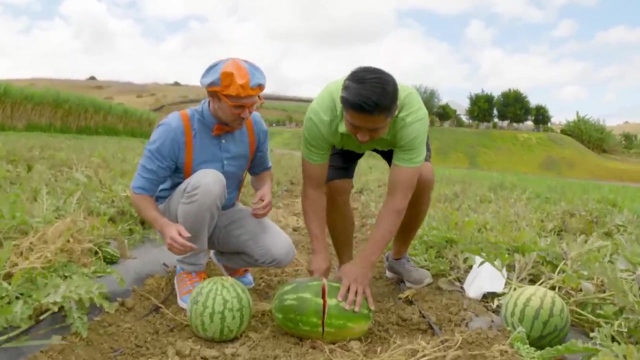 Yeah, Okay, wow, These are so nice. Okay, all right, So this is a normal watermelon and we know what the color inside is, but we should just cut it open and check, right. Let's see what it looks like. 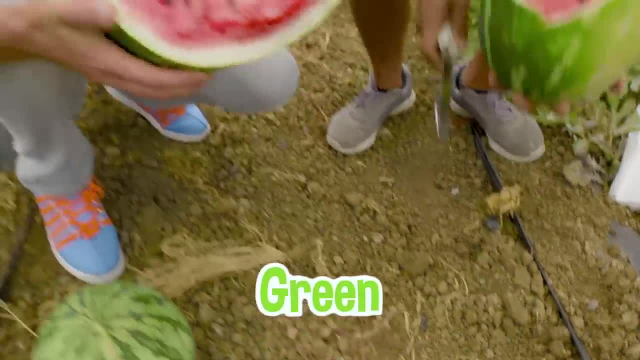 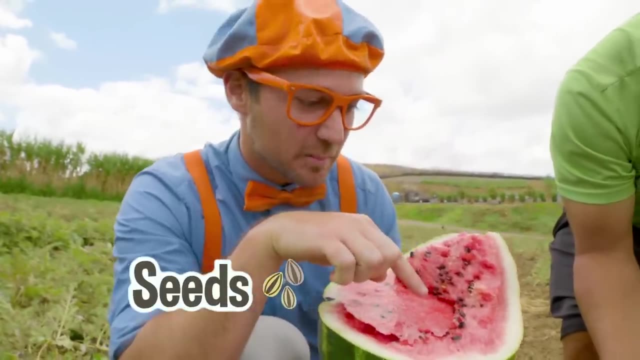 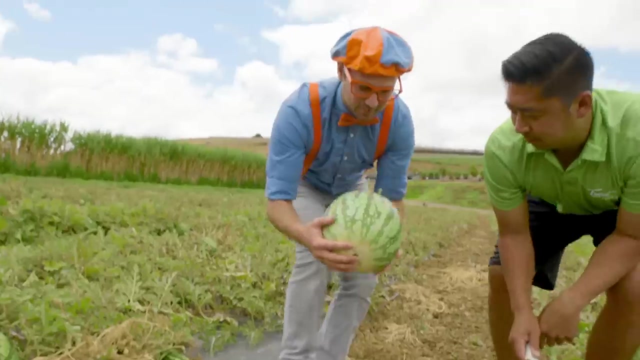 Wow, yeah, Green on the outside and reddish, pink, red on the inside. Wow, And do you see the seeds? They're black seeds and white seeds. Whoa, okay, But since this watermelon looked a little different, what's so different about it? 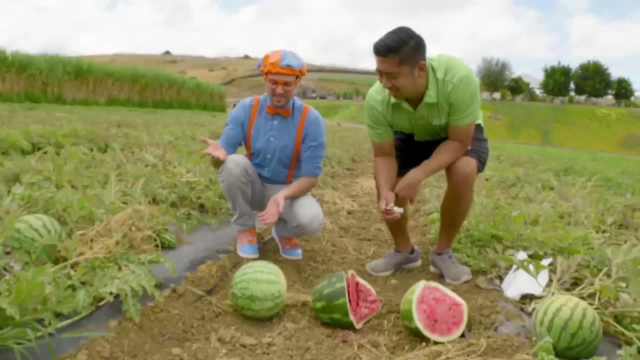 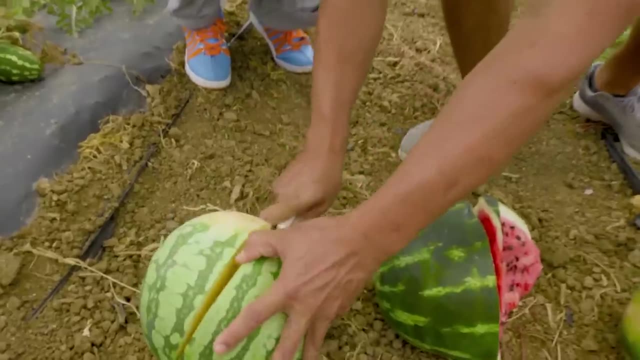 It just has a yellow inside flesh. Oh, that makes sense. Yeah, because it's called a yellow watermelon. Can we cut it open? Yeah, let's cut it open and see. When they're nice and ready, they pop right open. 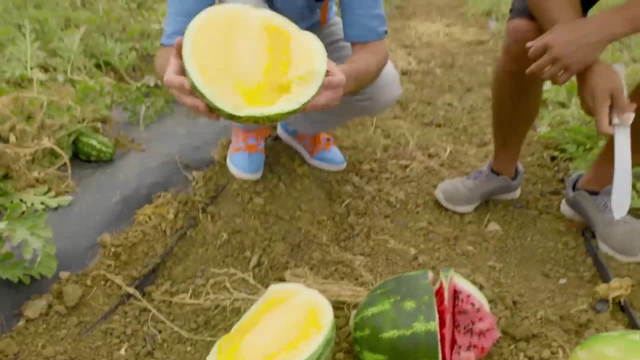 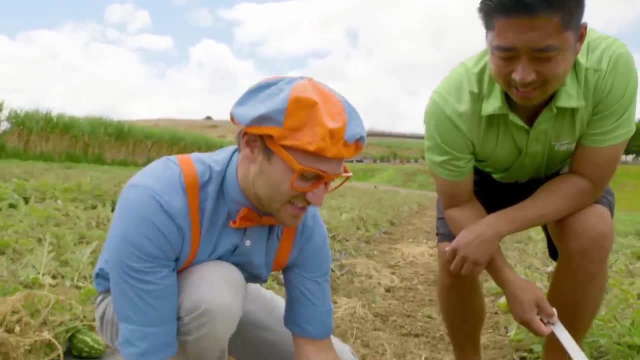 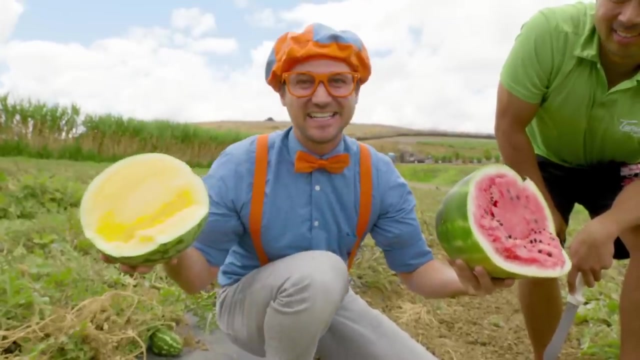 Yeah, Whoa. I've never seen a watermelon like this before. Look, This is the color yellow. Wow. All right, let's compare them. Yellow red, Yellow red- Both are tasty. Wow, Let's see how it tastes. 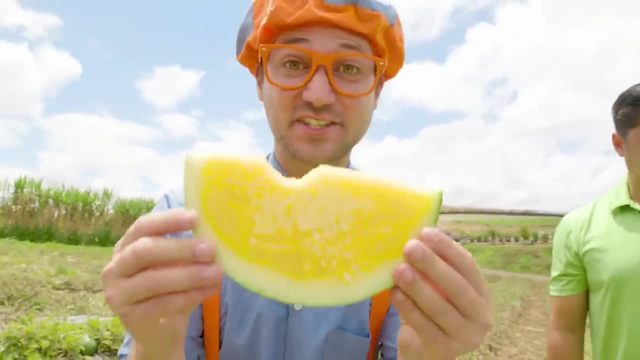 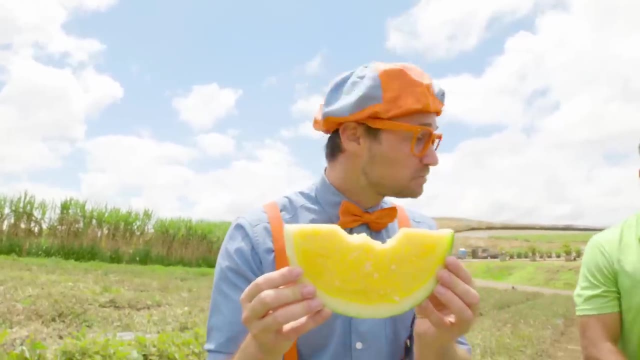 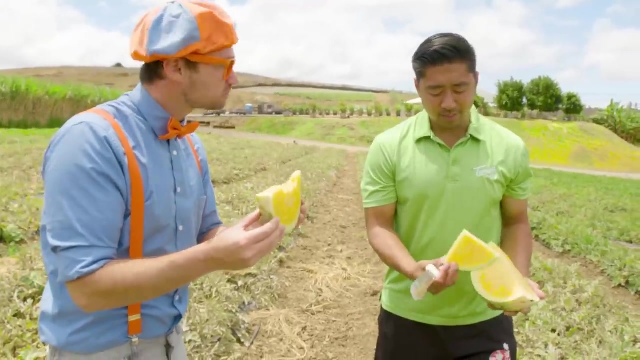 Mm Mm. that's sweet. I love the taste of yellow watermelon. Mm. mm. What color is your favorite of watermelon? My favorite is yellow. Mm Has a little bit different taste but tastes really good. 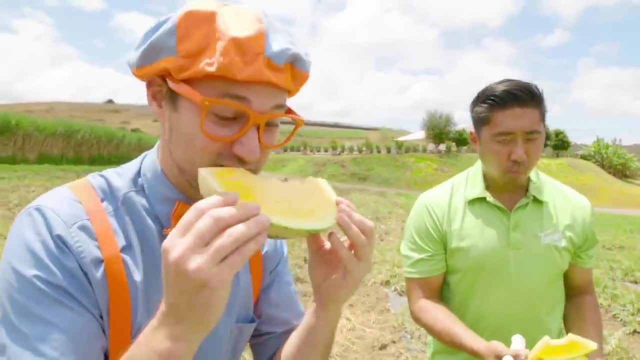 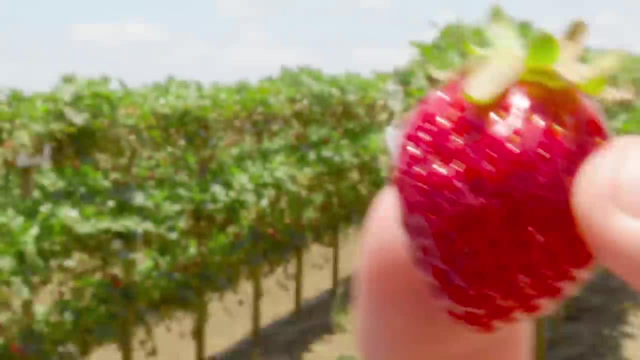 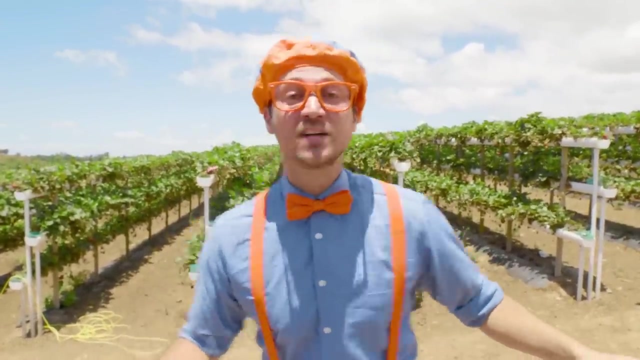 Mm-hmm. Yeah, let me tell you, This tastes really good. Mm-hmm, You want to try? Ooh, strawberry, Mm, Mm, Mm. Strawberries are so tasty, Let's go pick some more strawberries. 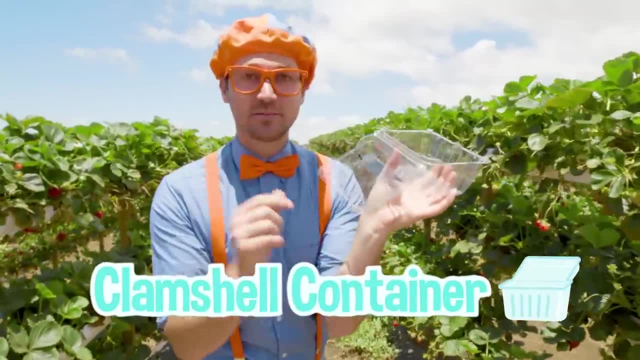 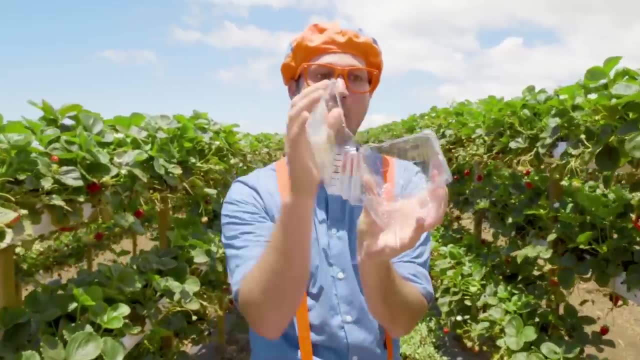 OK, Do you see my container? This is called a clam shell container. Yeah, Do you know what a clam is? Yeah, a clam is a shellfish and this kind of looks like it. Oh, oh, oh. OK, let's pick 20 strawberries. 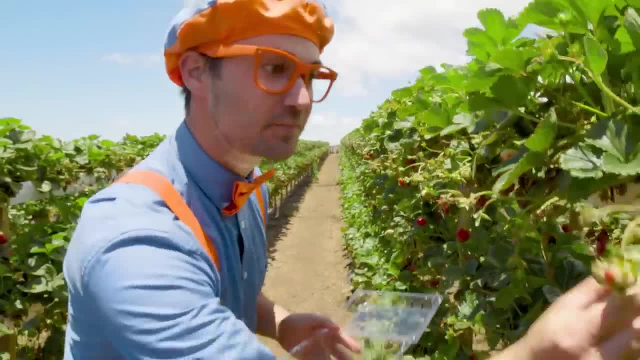 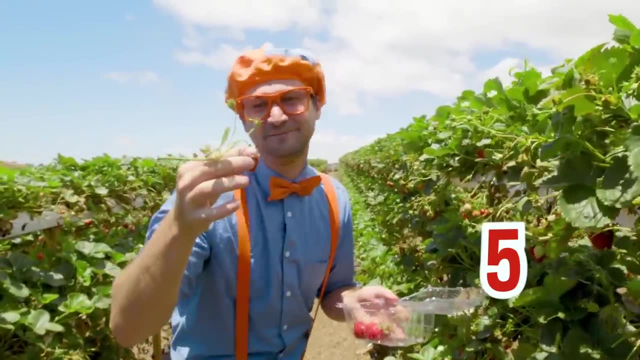 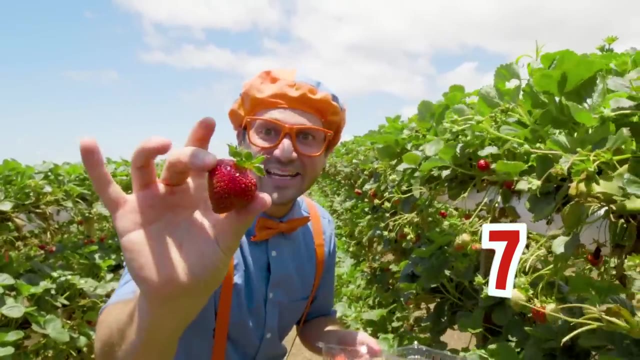 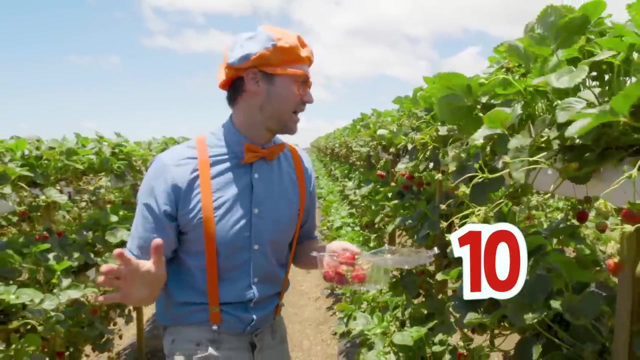 Whoa, that's a lot of strawberries. OK, ready. 1, 2,, 3,, 4,, 5,, 6,, 7,, wow, 8,, 9,, 10 strawberries. OK, we're halfway there. 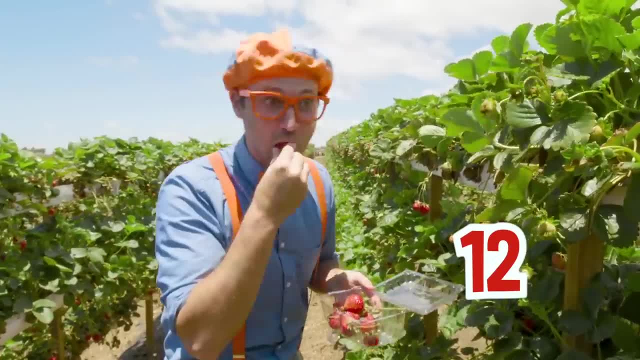 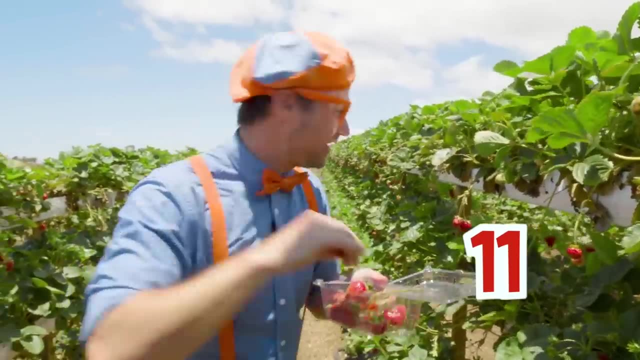 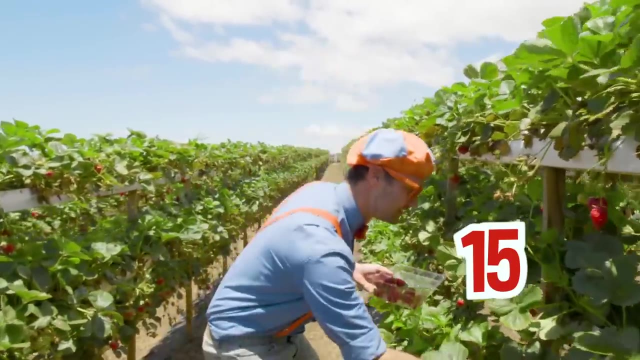 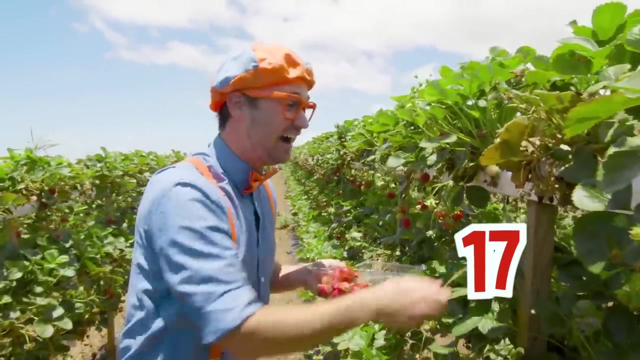 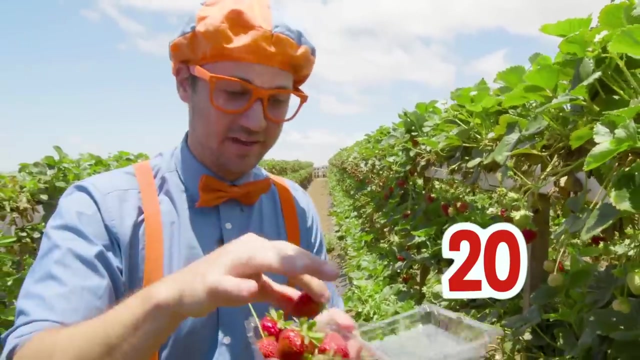 11,, 12, minus 1.. 11.. 12,, 13,, 14,, 15,, 16,, 17,, almost there, 18, 19.. Last one: 20, 20 strawberries in our clam shell container. 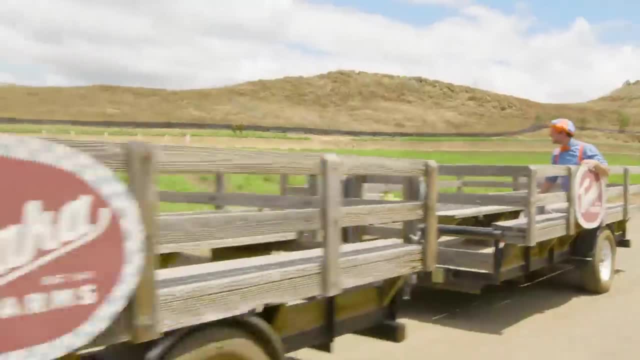 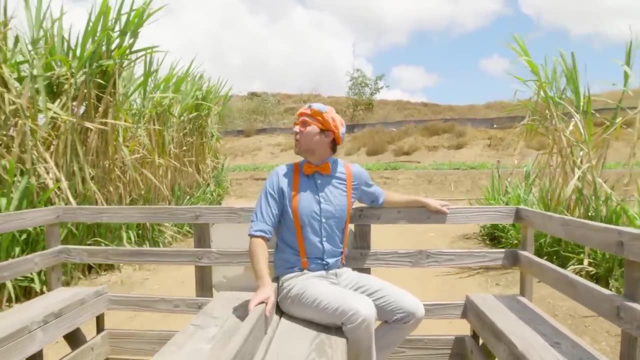 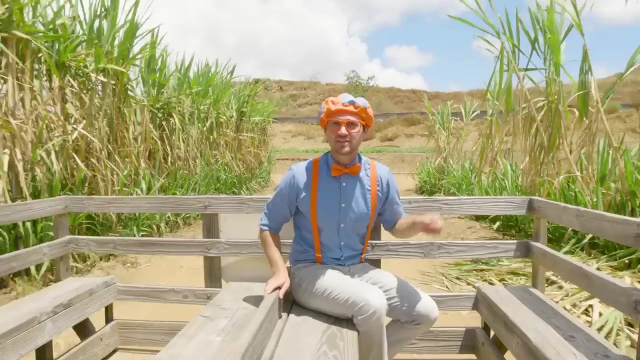 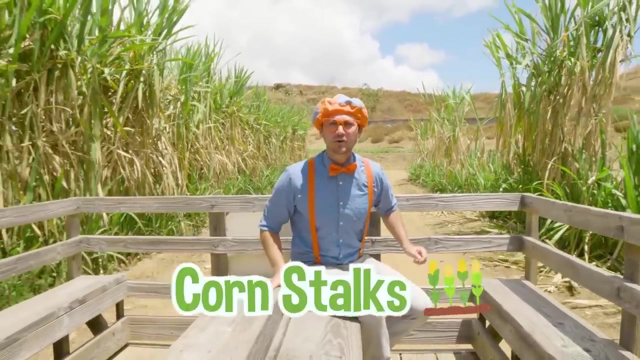 Good job. Ha ha, ha, Woo-hoo. Wow, What kind of plants are these? I've never seen these before. Wow, Look at them. They're so tall. Kind of looks like corn stalks, but I know they're not corn stalks. 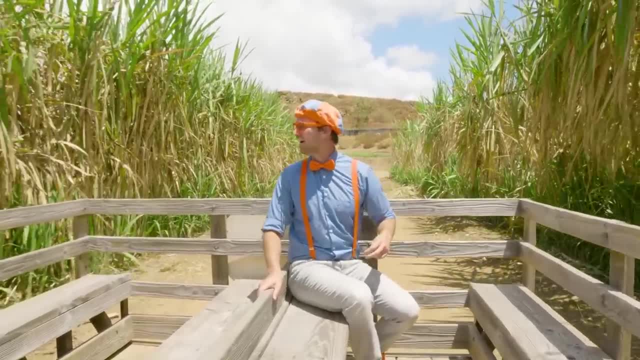 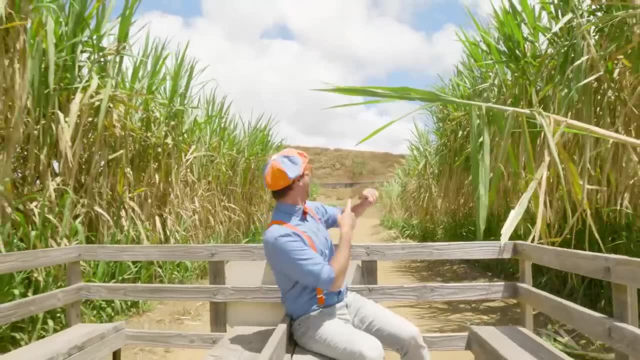 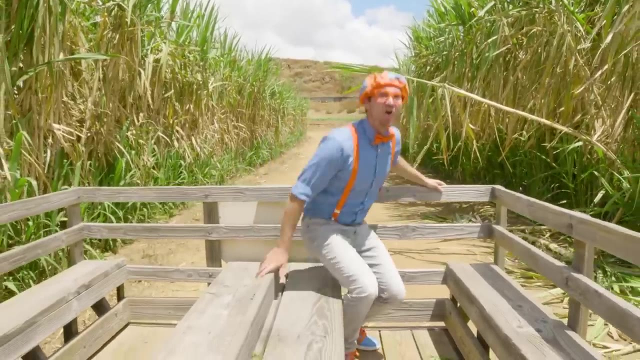 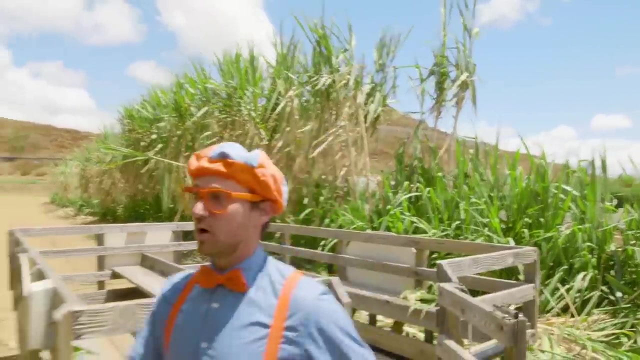 Wow, Whoa, whoa, ha ha, That almost hit me. Ha ha, We're stopping. All right, Blippi, we're here on sugarcane lane. Sugarcane lane, Did you hear that? Oh, that's what these must be: sugar canes. 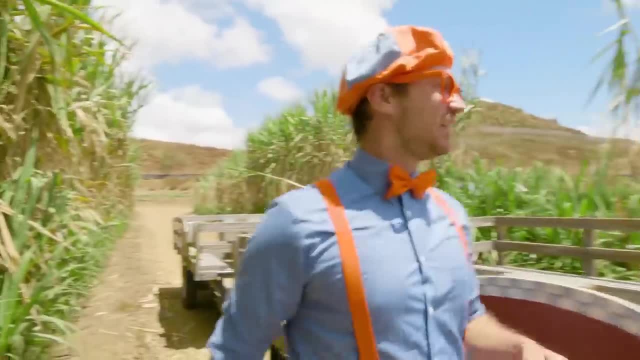 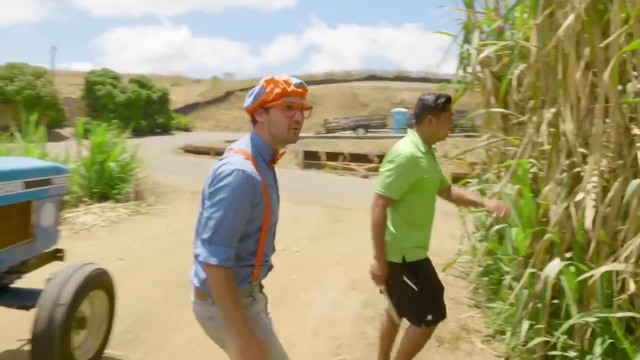 Whoa, OK, All right, Farmer Kenny. OK, All right, All right. What do we do now? We're going to cut some sugarcane down. OK, Wow, Hey, these are sugarcane. Look for a nice stalk. 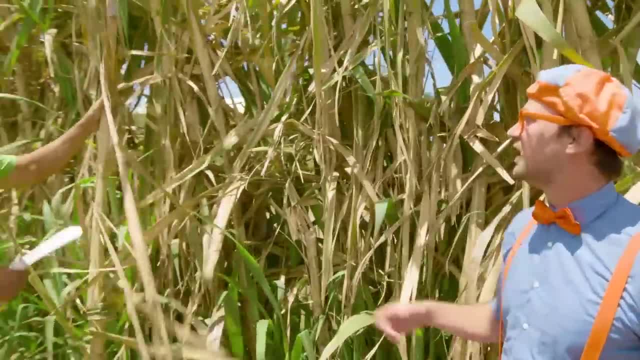 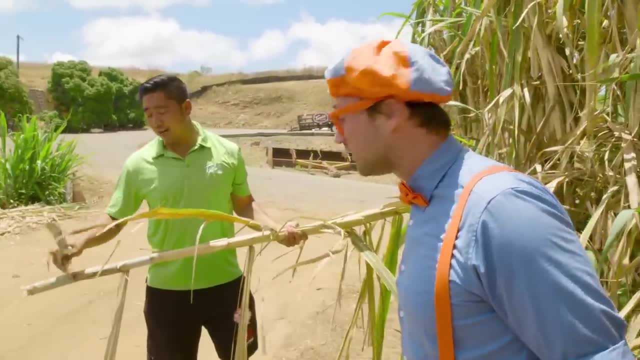 Whoa, Whoa, that's a sharp knife, Ha ha, He just chopped it down. Wow, what's sugarcane used for? You could use it just to suck on. You could use it to press it out and make juice out of it. 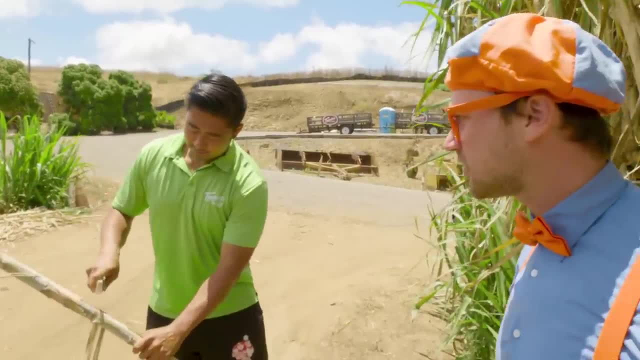 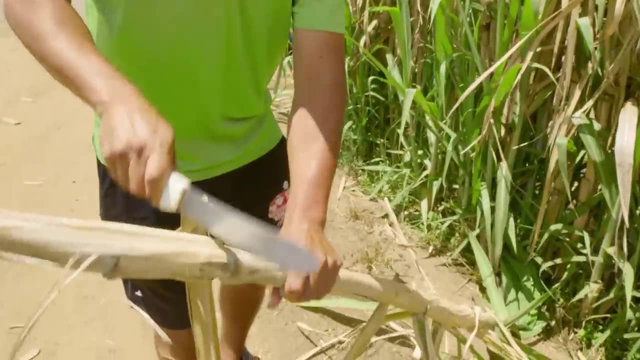 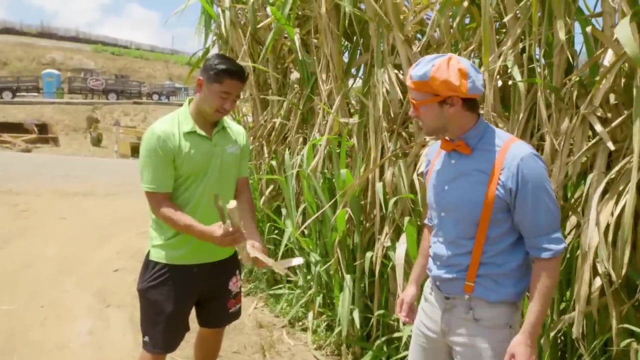 Ooh, Cook with it. Is that what they make sugar out of? Yeah, Whoa, Sugarcane makes sugar. Wow, OK, Wow, look at that. So normally you just cut off the skin and chew on the inside. 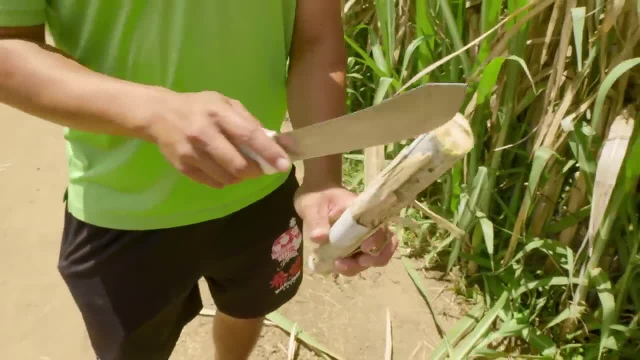 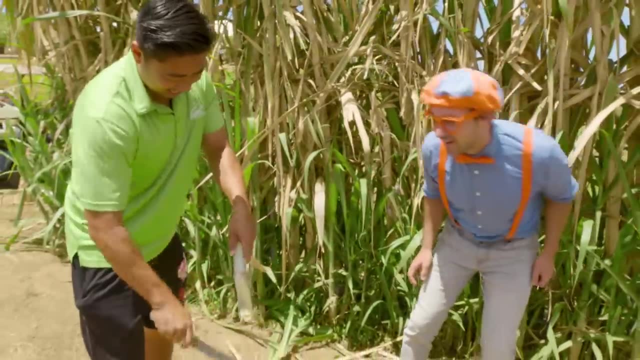 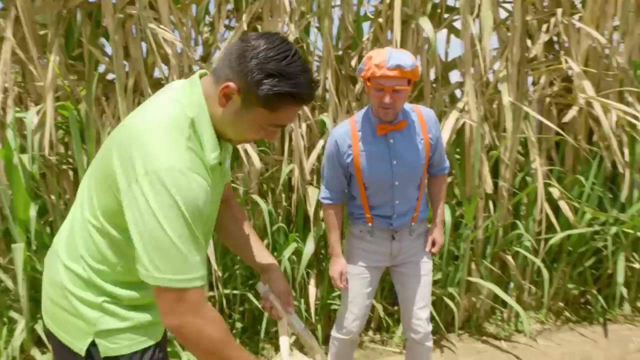 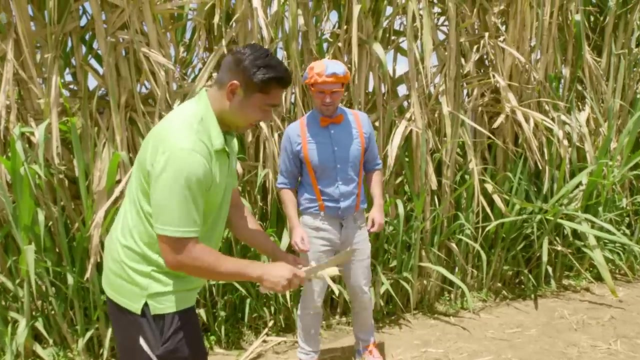 Wow, So you can chew on that right there. Yeah, OK, Wow. Any time you use a knife, you have to be very careful. right, grown-ups, And only grown-ups, can use a knife. Oh, all right, That looks so yummy. 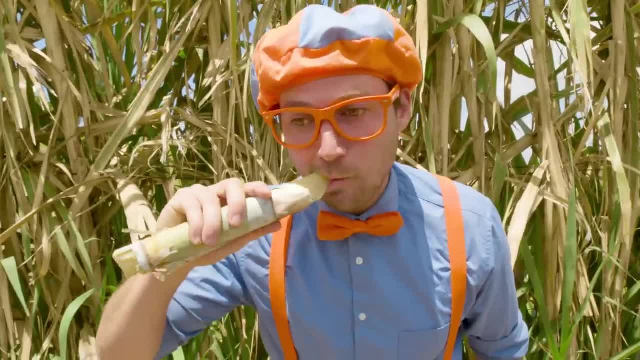 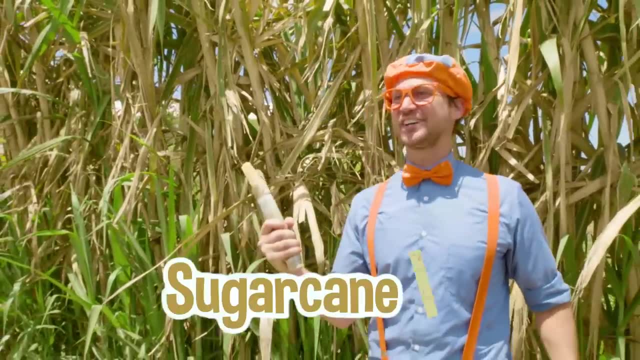 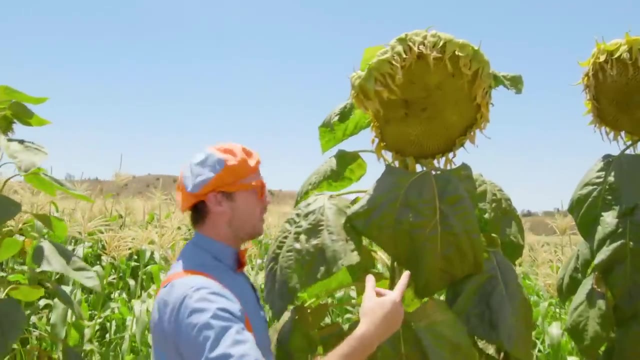 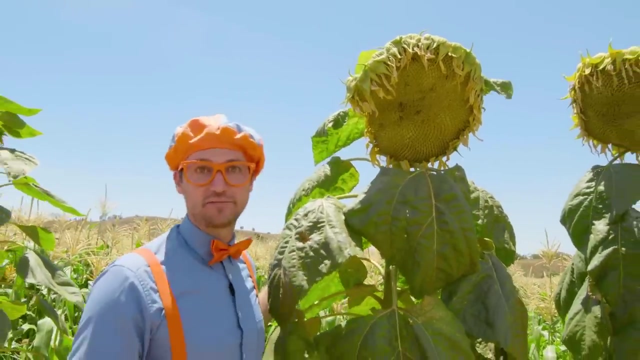 Could chew on that little end. All right, let's try it. Mm, Mm, I love sugarcane. Whoa, Check this out. Whoa, This is a monstrous plant And this is actually a flower. This is a giant flower. 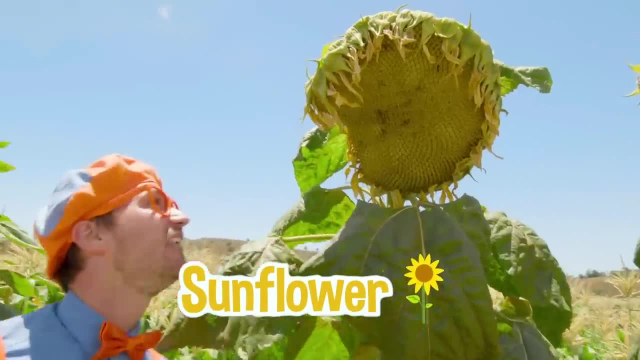 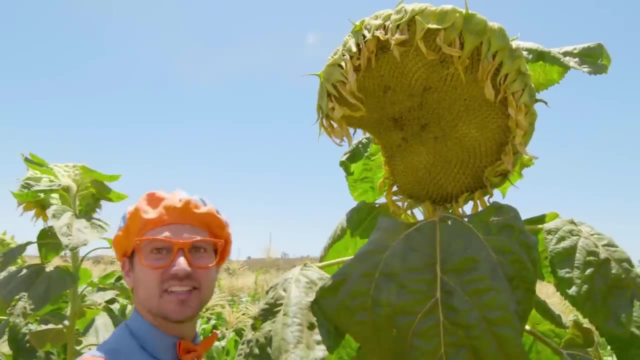 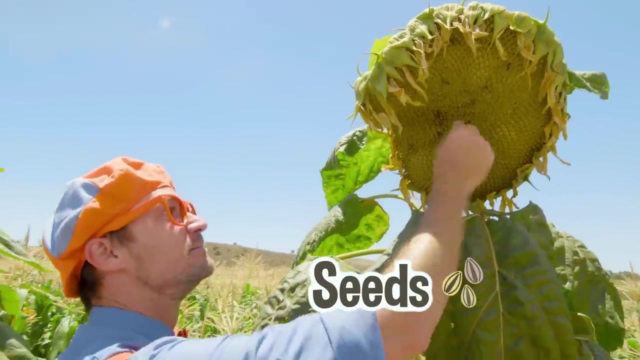 And this flower is called a sunflower. Wow, Can you tell why it's called a sunflower? Yeah, Because it looks like the sun. Whoa, Wow, And sunflowers produce seeds. Hm, Hm, Hm. 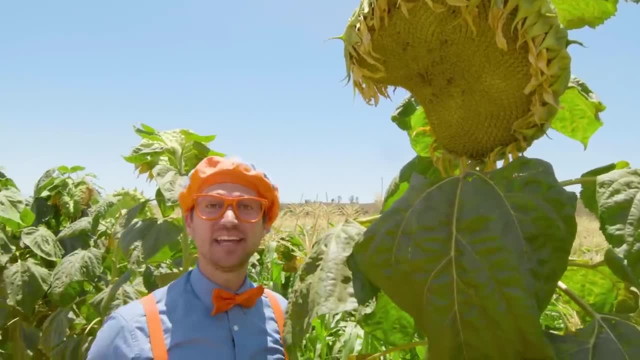 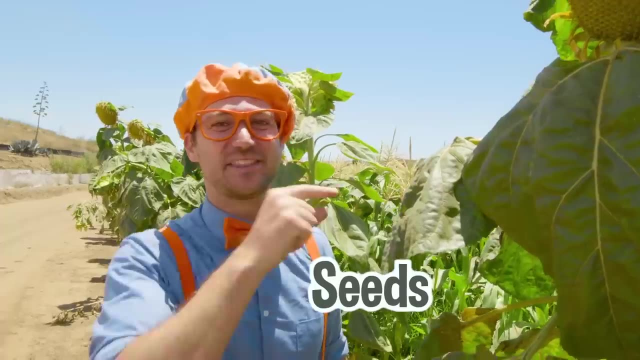 Hm, Hm, Hm, Yummy Seeds are really healthy. Well, this has been so much fun learning about fruits, vegetables and seeds with you at Tanaka Farms in Irvine, California. Well, this is the end of this video. 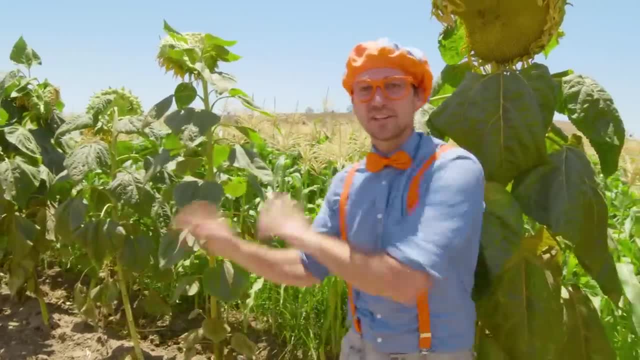 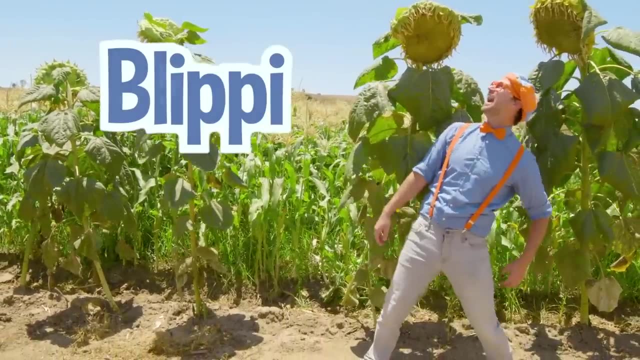 But if you want to watch more of my videos, all you have to do is search for my name. Will you spell my name with me? Ready, B-L-I-P-P-I, Blippi, Good job, All right, See you later. Buh-bye.